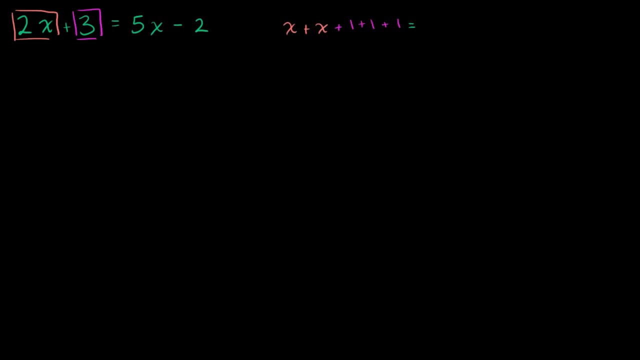 And then that is equal to 5x's. I'll do that again In blue: That is equal to 5x's. So 1,, 2,, 3,, 4,, 5.. And I want to make it clear. 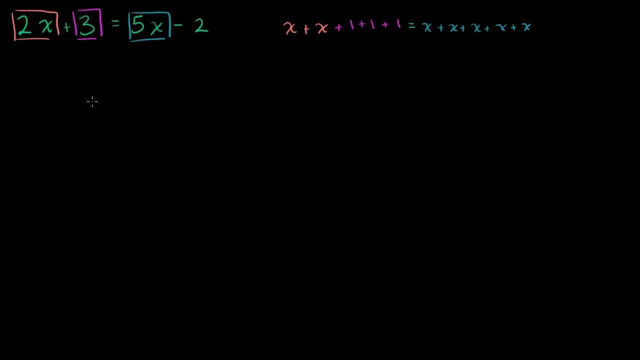 You would never actually have to do it this way when you're solving the problem. You would just have to do the algebraic steps. But I'm doing this for you so you can actually visualize what this equation is saying. The left-hand side is these two orange x's plus 3.. 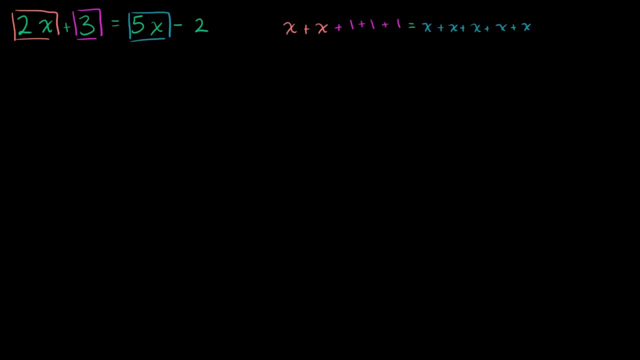 The right-hand side is 5x minus 2.. So minus 2. we could write as minus. Let me do this in a different color. I'll do it in pink. So minus 2. I'll do as minus 1 and minus 1.. 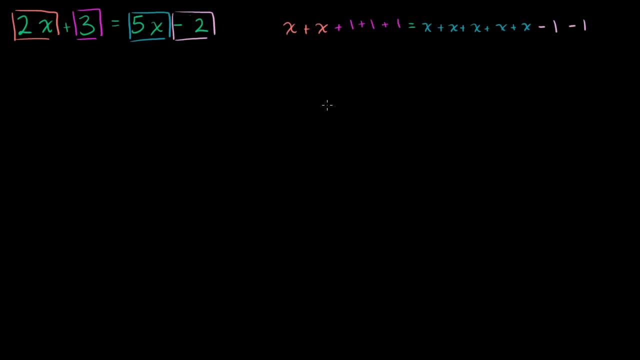 Now we want to isolate the x's on the same side of the equation. So how could we do that? Well, there's two ways of doing it. We could subtract these two x's from both sides of the equation, And that would be pretty reasonable. 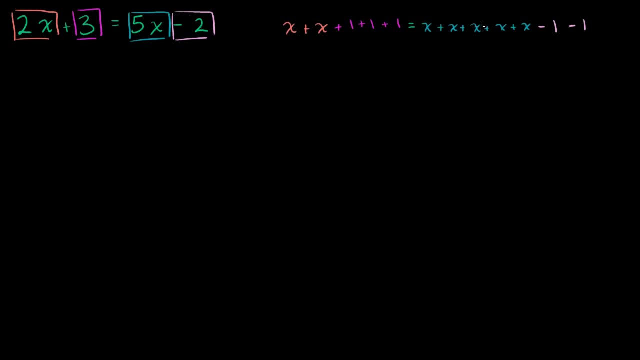 Because then you'd have 5x's minus the 2x's, You'd have a positive number of x's on the right-hand side, Or you could actually subtract 5x from both sides. And that's what's neat about algebra. 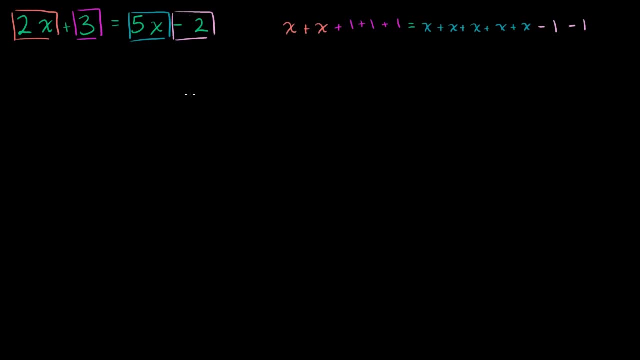 As long as you do legitimate operations, you will actually get the right answer. So let's just start off subtracting 2x from both sides of the equation, And when I mean that, I mean we're going to remove 2x's from. 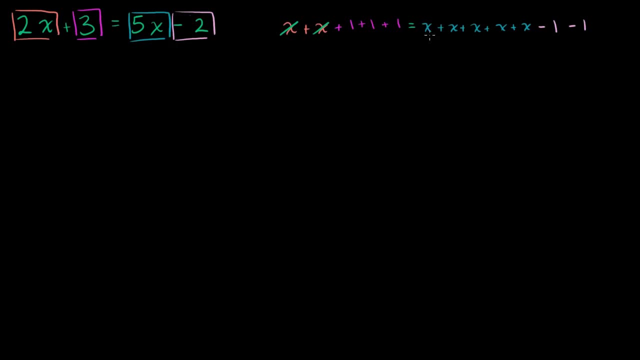 the left-hand side. And if we remove 2x's from the left-hand side, we have to remove 2x's from the right-hand side, Just like that. So what does that give us? We're subtracting 2x's from the left. 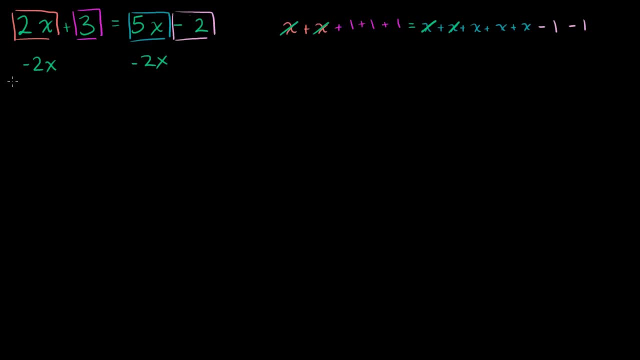 And we're also going to subtract 2x's from the right. Now what does our left-hand side simplify to? We have 2x plus 3.. Minus 2x, The 2x's cancel out. So you're just left with the 3.. 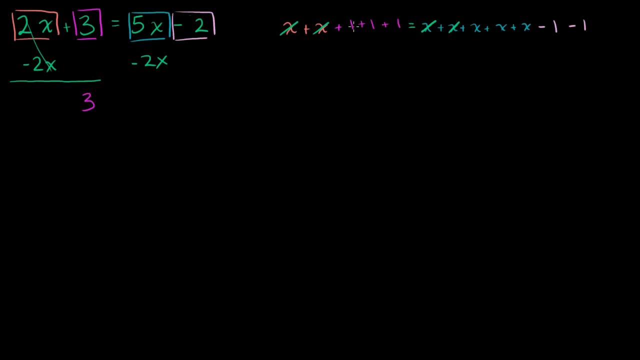 And you see that over here We took two of these x's away. We're just left with the plus 1, plus 1, plus 1.. And then, on the right-hand side, 5x minus 2x. We have it over here. 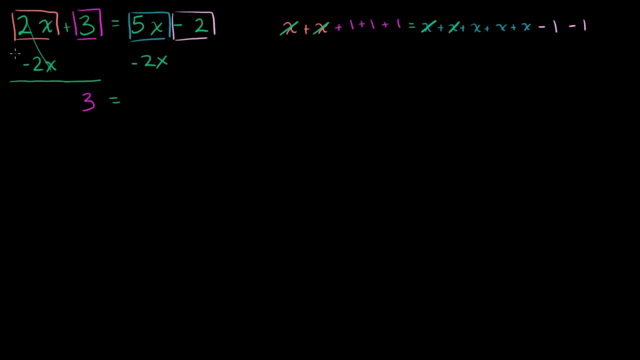 We have 5x's minus 2x's. You only have 1,, 2, 3x's left over. 3 is equal to 3x, And then you have your minus 2. there You have your minus 2x. 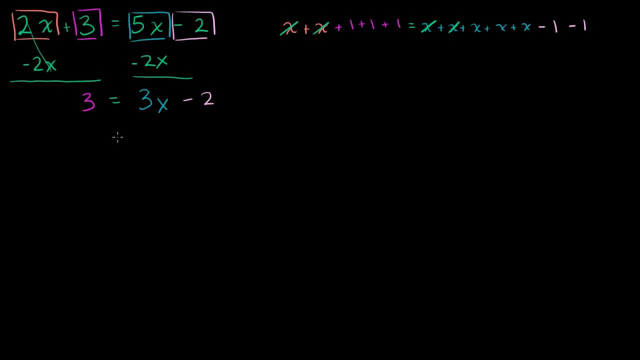 So normally, if you were to do the problem, you would just have to write what we have here on the left-hand side. So what can we do next? Remember, we want to isolate the x's. Well, we have all of our x's on the right-hand side, right here. 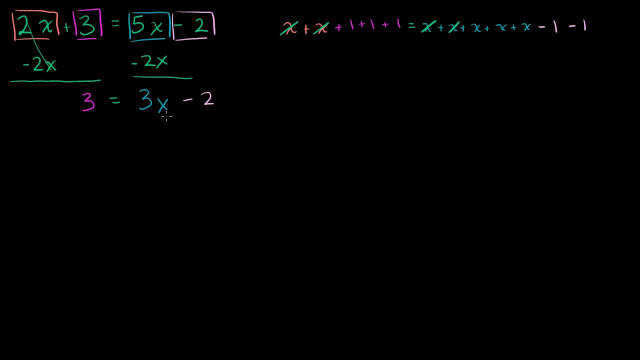 If we could get rid of this negative 2 off of the right-hand side, then the x's will be alone, They'll be isolated. So how can we get rid of this negative 2?? Or, if we visualize it over here, this negative 1, this negative. 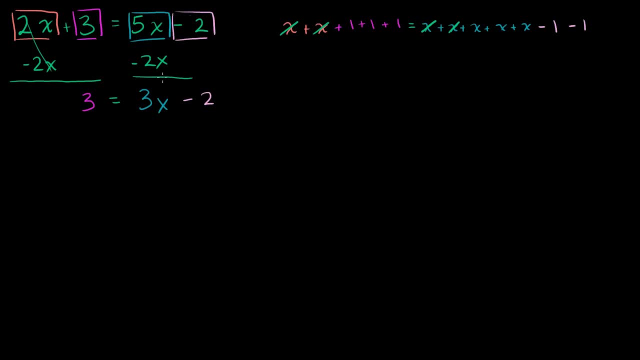 1?? Well, we could add 2 to both sides of this equation. Think about what happens there. So if we add 2.. So I'm going to do it like this: 1 plus 1.. So you can literally see we're adding 2.. 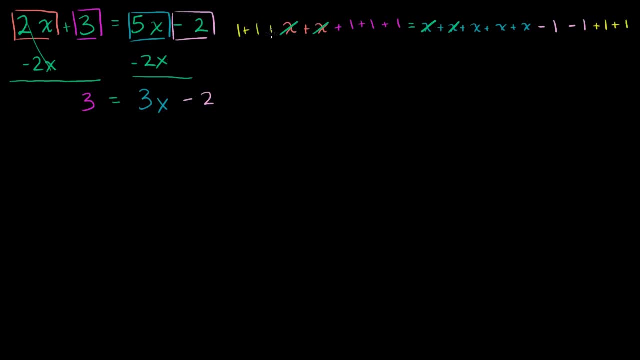 And then we're going to add 2 to the left-hand side. 1 plus 1, plus What happens. Let me do it over here as well. So we're going to add 2.. We're going to add 2.. 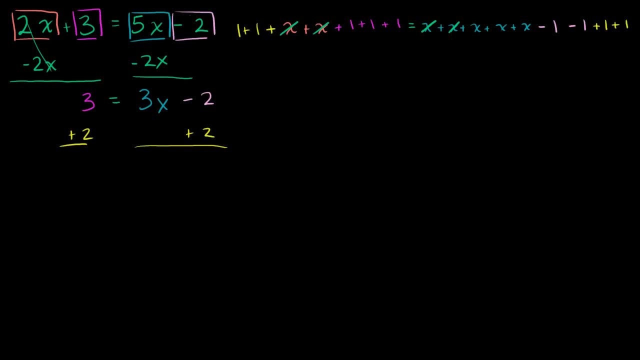 So what happens to the left-hand side? 3 plus 2 is going to be equal to 5. And that is going to be equal to 3x minus 2 plus 2.. These guys cancel out and you're just left with 3x. 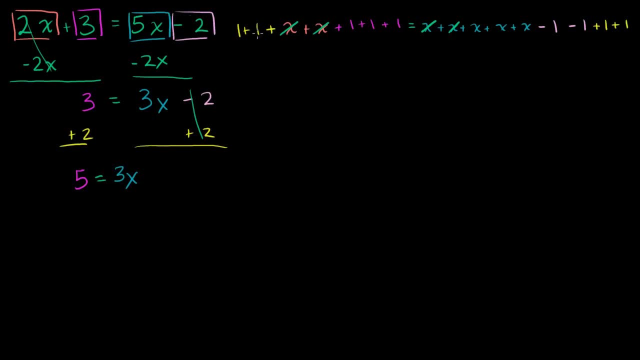 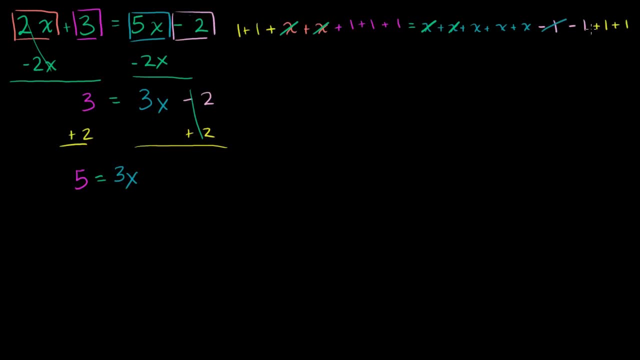 And then we have the negative 1, negative 1, plus 1, plus 1.. Negative 1, these cancel out. They get us to 0.. They cancel out. So we're just left with: 5 is equal to 3x. 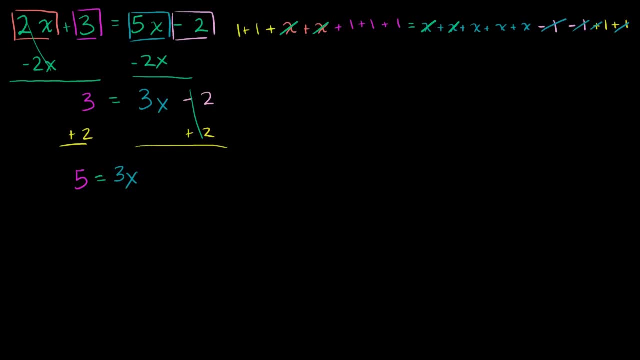 So we have 1,, 2,, 3,, 4,. 5 is equal to 3x. Let me clear everything that we've removed so it looks a little bit cleaner. Let me clear that out, And then let me clear. 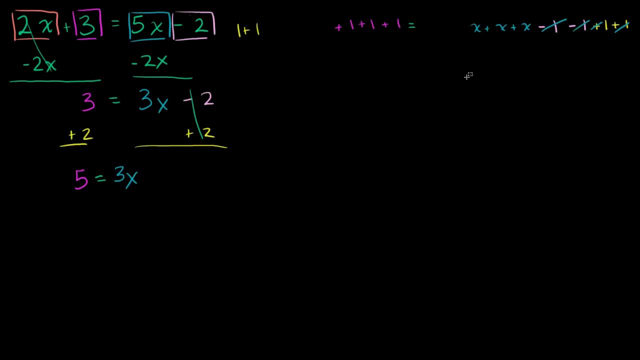 These are all of the things that we've removed. Let me clear that out And then let me clear that out like that. Edit clear. So now we are just left with 1,, 2,, 3,, 4, 5.. 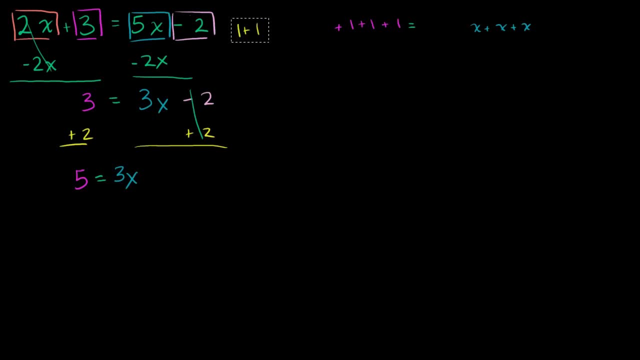 Actually let me move this over. So edit cut, Edit paste, So I could just move this over right over here. We now have 1,, 2,, 3,, 4, 5.. These are the two that we added here. 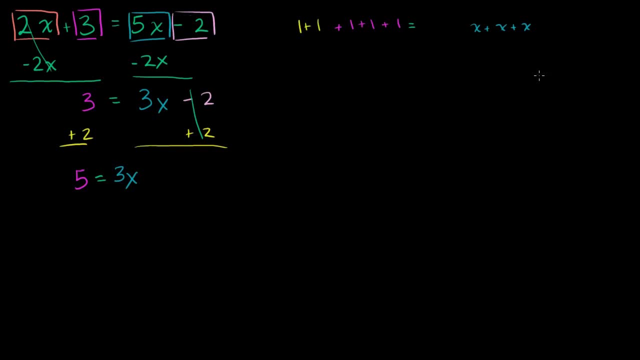 It's equal to 3x. These guys canceled out. That's why we have nothing there Now to solve this. we just divide both sides of this equation by 3. And this is going to be a little hard to visualize over here. 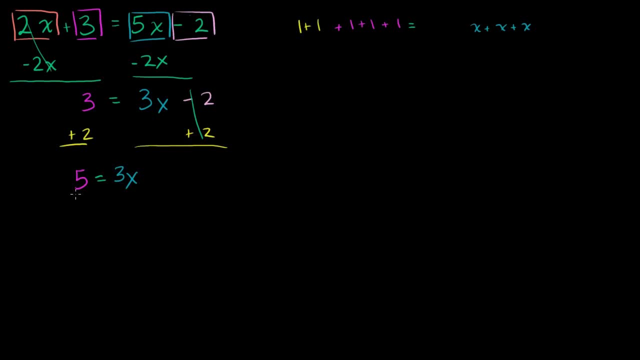 But if we divide over here both sides by 3, what do we get? We divide the left by 3.. We divide the right by 3.. The whole reason why we divided by 3 is because the x was being multiplied by 3.. 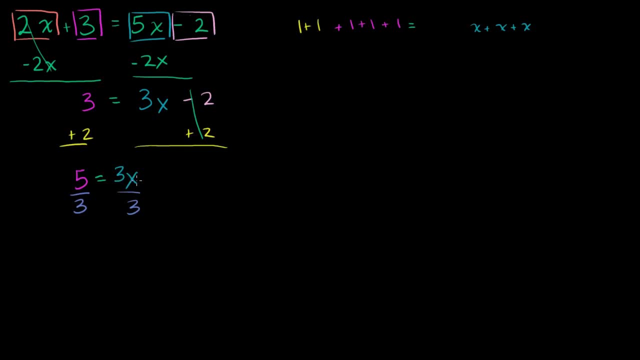 3 is the coefficient on the x Fancy word. it literally just means the number multiplying the variable, The number we're solving, the variable we're solving for. So these 3's cancel out The right-hand side of the equation is just x. 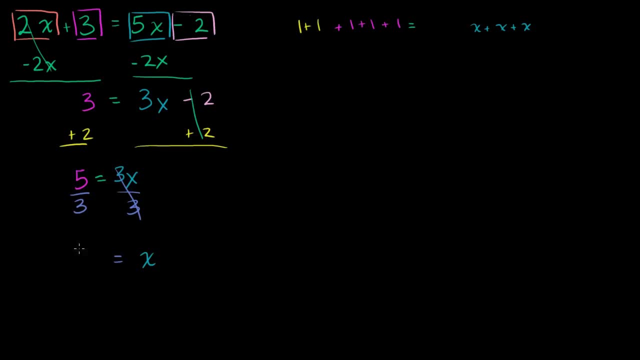 The left-hand side is 5 thirds. So 5 thirds, we could say x is equal to 5 thirds And this is different than everything we've seen so far. I now have the x on the right-hand side, the value on the left-hand side. 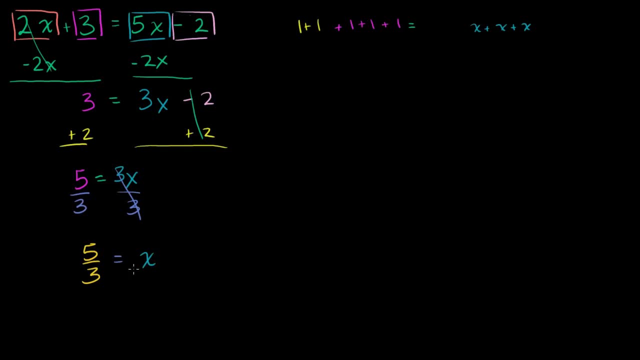 That's completely fine. This is the exact same thing as. saying 5 thirds is equal to x is the same thing as saying x is equal to 5 thirds- Completely equivalent. Completely equivalent. We sometimes get more used to this one, but this is completely the same thing. 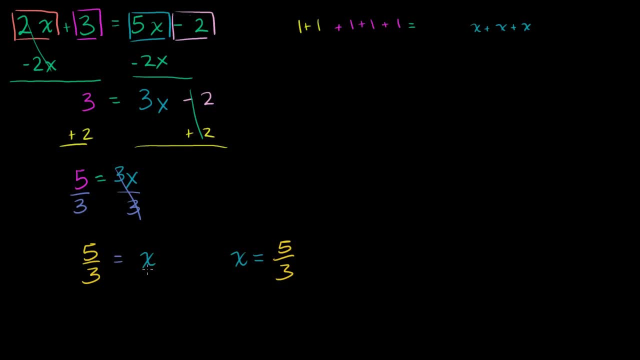 Now, if we wanted to write this as a mixed number, 3 goes into 5 one time with remainder 2.. So it's going to be 1 and 2 thirds. So we could also write that x is equal to 1 and 2 thirds. 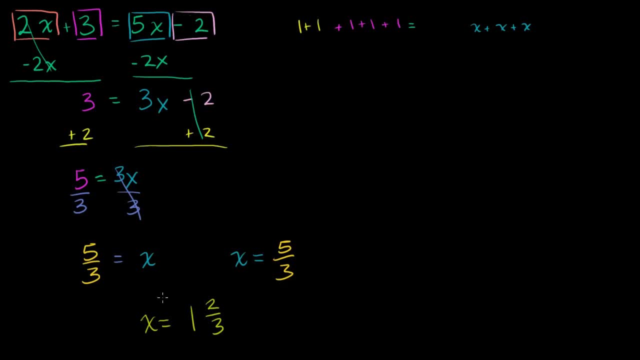 And I'll leave it up for you to actually substitute back into this original equation and see that it works out. Now, to visualize it over here: how did you get 1 and 2 thirds? Let's think about it. Instead of doing 1,, I'm going to do circles. 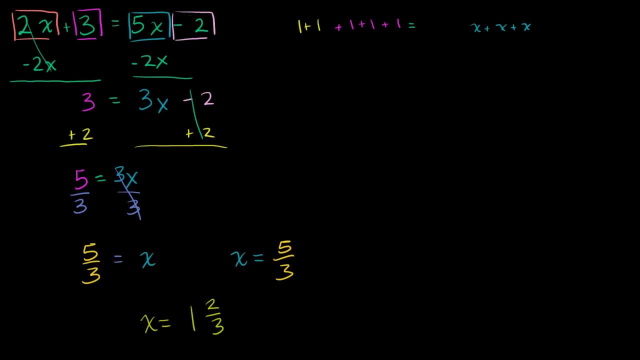 I am going to do circles. Actually, even better, I'm going to do squares. So I'm going to have 5 squares on the left-hand side. I'll do it in this same yellow color right here. So I have 1,, 2,, 3,, 4,, 5.. 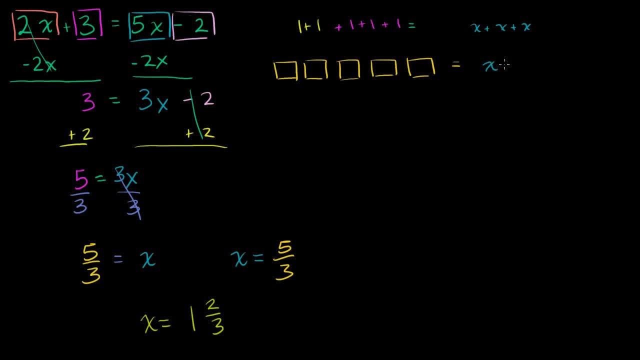 And that is going to be equal to the 3 x's: x plus x plus x. Now we're dividing both sides. We're dividing both sides of the equation by 3.. Actually, that's what we did up here. We divided both sides by 3.. 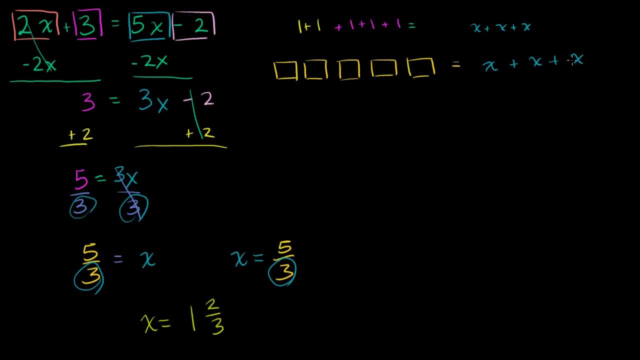 So how do you do that? Right-hand side is pretty straightforward. You want to divide these 3 x's into 3 groups, That's 1, 2, 3 groups: 1, 2, 3.. Now how do you divide 5 into 3?? 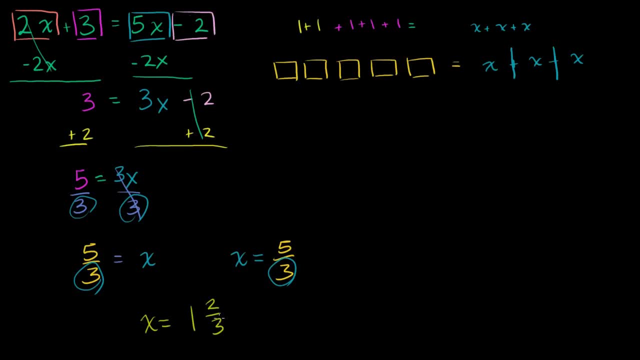 And they have to be even groups. And here the answer tells us: each group is going to be 1 and 2 thirds. So 1 and 2 thirds, So it's going to be 2 thirds of this next one, And then we're going to have 1 and 2 thirds. 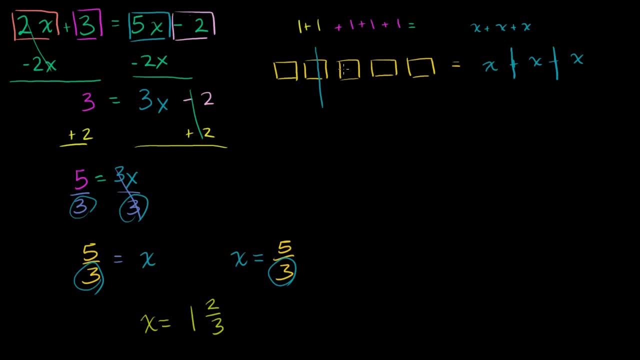 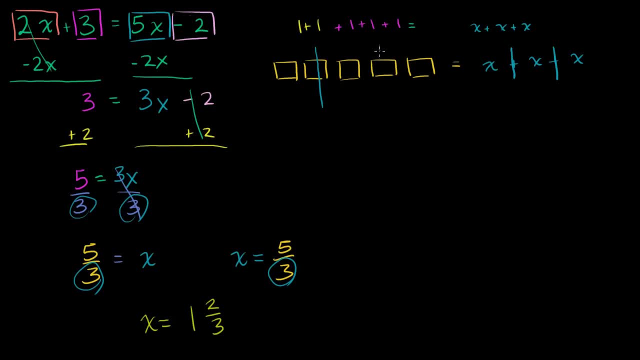 So this is 1 and 1 third. We're going to need 1 more third, So it's going to be right here, And then we're left with 2 thirds and 1.. So we've broken it up into 3 groups. 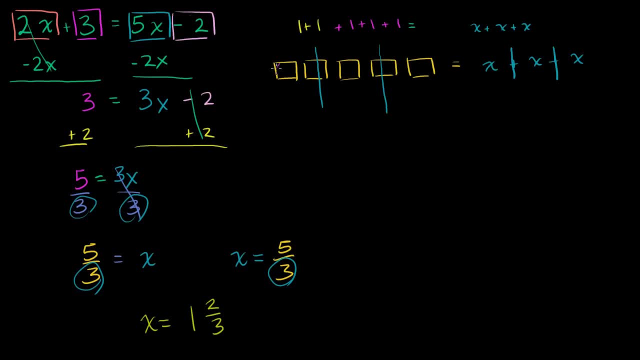 This right here, let me make it clear: This right here is 1 and 2 thirds, And then this right here: this is 1 third, That's another 1 third, So that's 2 thirds, And then that's 1 right there. 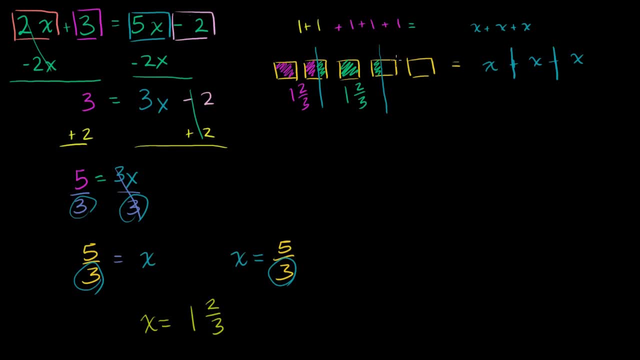 So that's 1 and 2 thirds. And then finally, this is 2 thirds And this is 1.. So this is 1 and 2 thirds. So when you divide both sides by 3, you get 1 and 2 thirds. 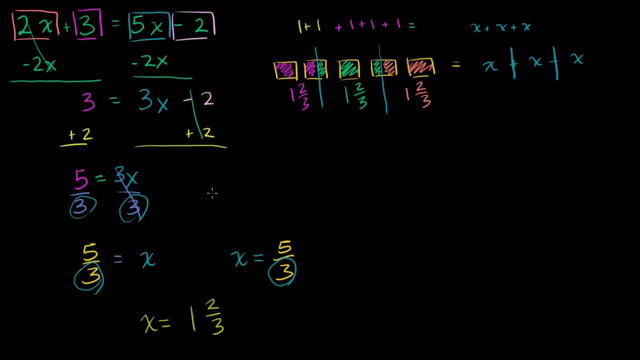 Each section, each bucket is 1 and 2 thirds on the left-hand side, or 5 thirds, And on the right-hand side we just have an x. So it still works A little bit harder to visualize with fractions.